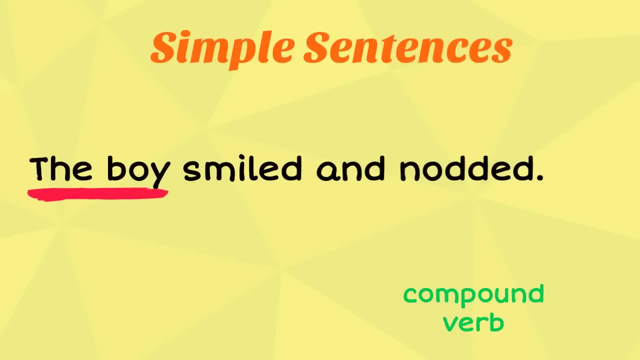 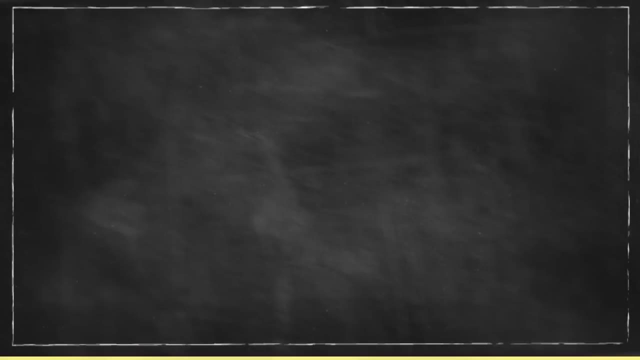 also have a compound verb. For example, the boy smiled and nodded. Here is another simple sentence. Even though it's longer, we know it's still a simple sentence because it has one subject and one verb: Compound sentences. Compound sentences are a combination of two or more independent clauses. 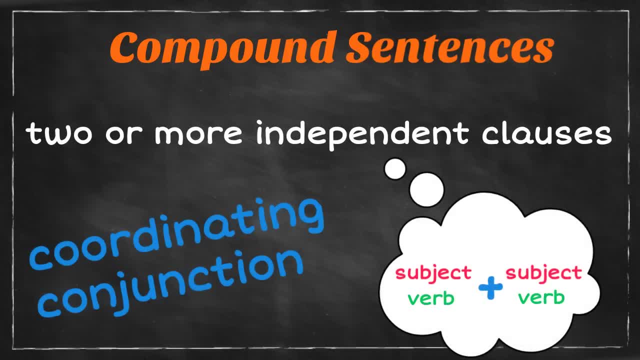 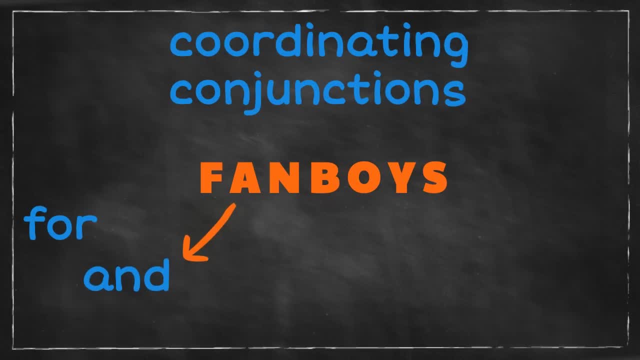 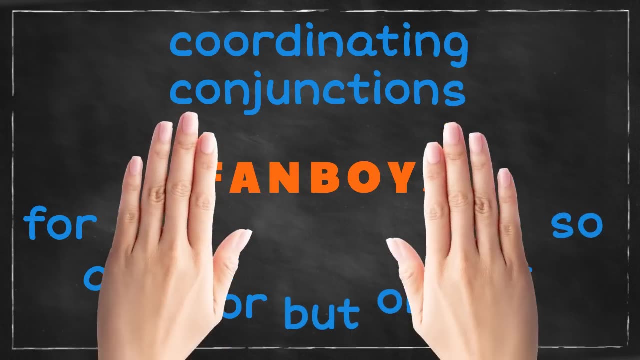 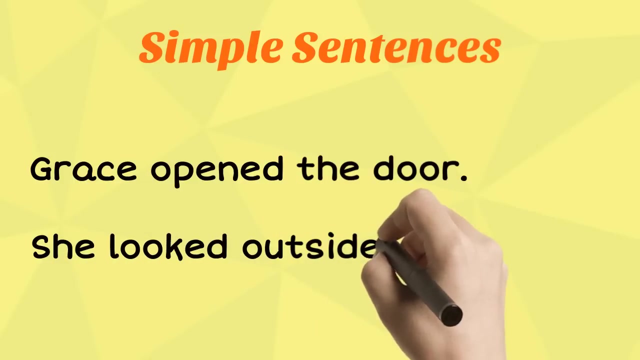 joined together by a coordinating conjunction. Remembering the acronym FANBOYS is an easy way to remember the coordinating conjunctions that we can use to join independent clauses. Here are two simple sentences, sentences: Grace opened the door. She looked outside. Let's join them using the coordinating. 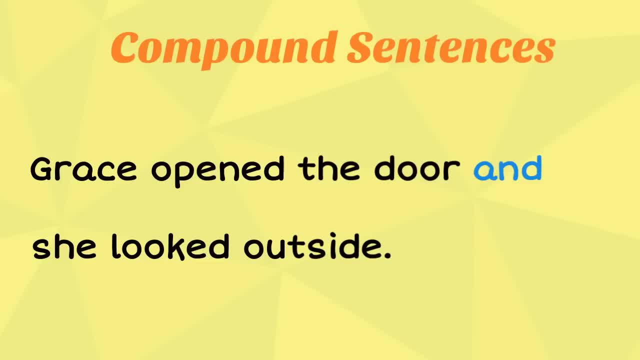 conjunction and We have created a compound sentence. Grace opened the door and she looked outside. The sentence has two independent clauses, That is, both clauses are a completed thought with a subject and a verb. Here are some other compound sentences. They each have more than one. 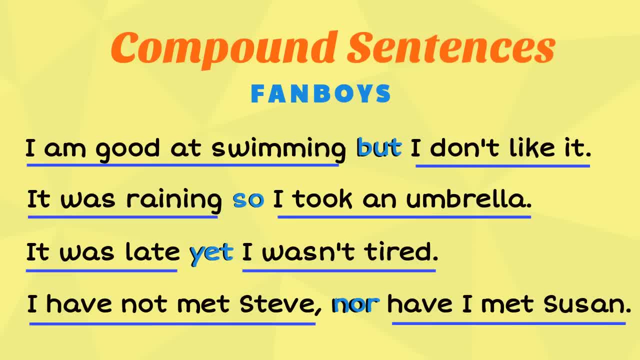 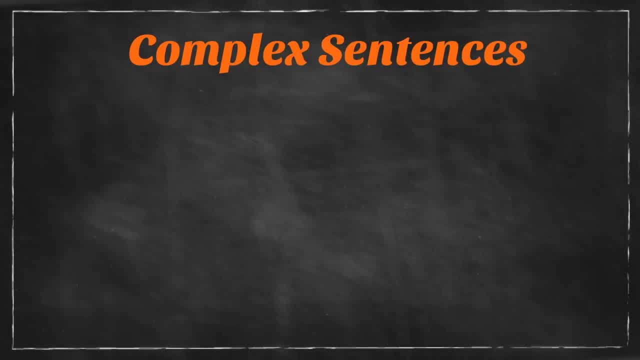 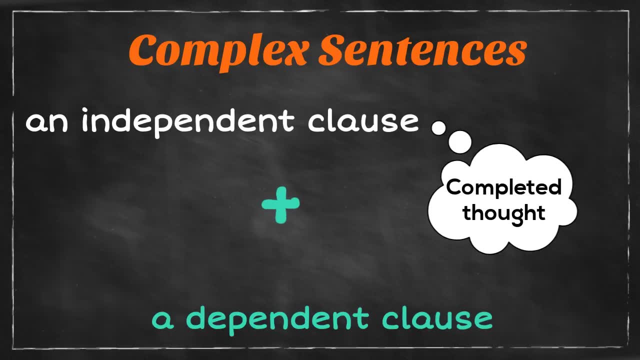 independent clause and are joined by a coordinating conjunction- Complex sentences. Complex sentences are composed of an independent clause and a dependent clause. Dependent clauses are not completed thoughts. Here is a compound sentence. Grace opened the door and she looked outside. Let's join them using the 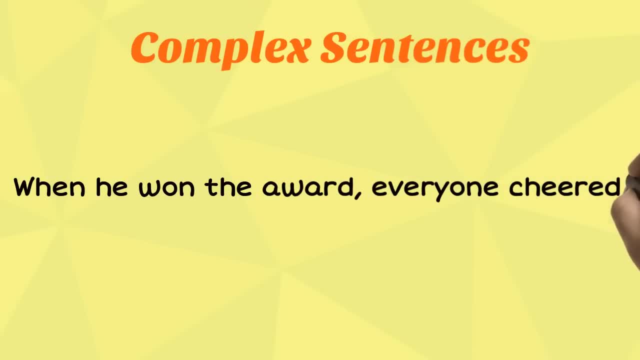 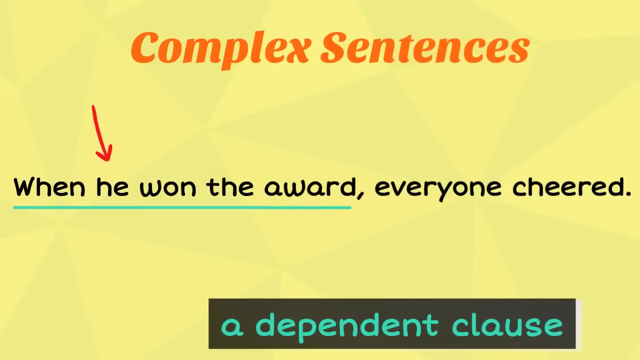 There is a complex sentence. When he won the award, everyone cheered. This is the independent clause because it has one subject and one verb and it's a completed thought. This clause is a dependent clause because, even though it has a subject and a verb, it's not a completed thought. 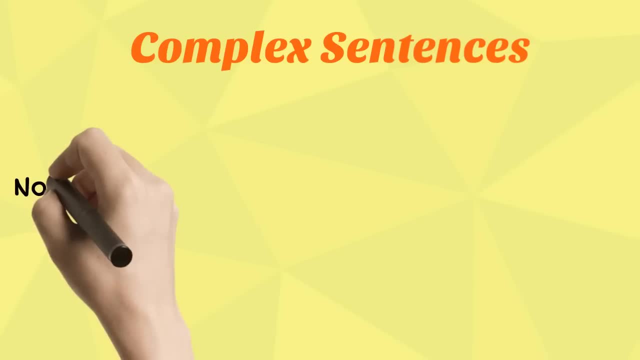 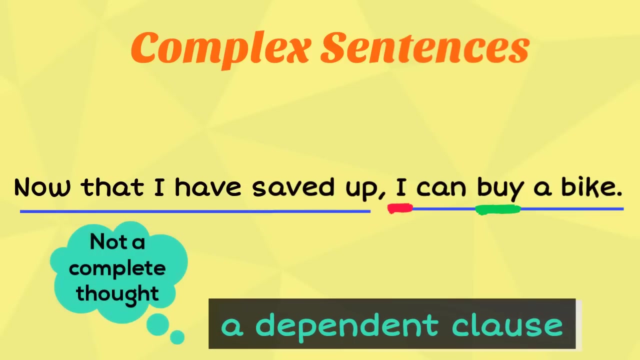 Let's look at another example. Now that I have saved up, I can buy a bike. This is an independent clause because it has one subject and one verb and it's a completed thought. Let's look at another example. Now that I have saved up, I can buy a bike. This is an independent clause because it has one subject and one verb and it's a completed thought. This is a dependent clause because it's not a completed thought.